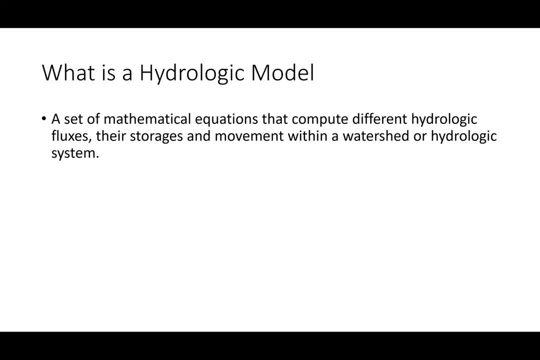 set of mathematical equations. In hydrology, these equations calculate or compute different hydrologic fluxes, their storages and movement within a watershed or hydrologic system. Most of these equations are conceptual. What that means is they may or may not truly represent a hydrologic process in the 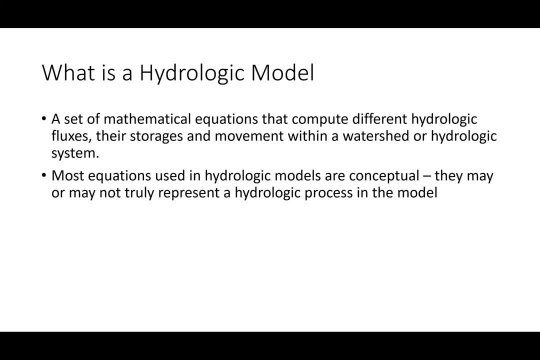 model, For example, we are familiar with curve number methods. so, as you know, a curve number doesn't really have any physical meaning or relevance within a watershed, but we still know that, what a higher curve number and lower curve number may mean. We also have equations. 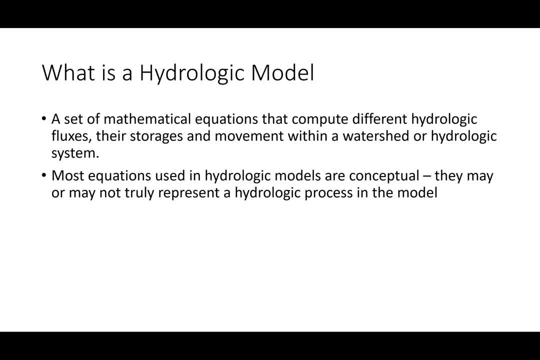 that are derived using physical laws and have physical meaning, but still those equations are derived using assumptions and many times those assumptions are not met in the hydrologic system, so they still may not truly represent a true process. However, all these equations are constrained to maintain the water balance or the continuity equation. What 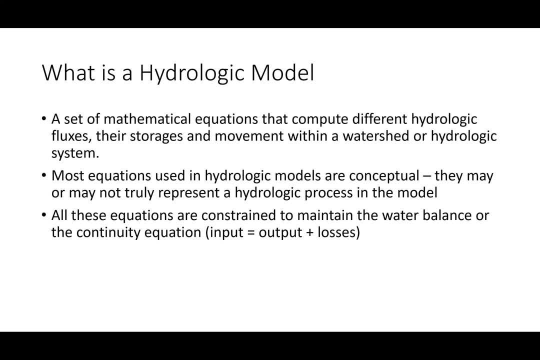 that means is that, regardless of what equations we are using in the model, the water balance still has to be maintained. so there is some physics involved there. All these equations have variables, or we call them parameters, and they also may or may not have a physical meaning in a hydrologic system. 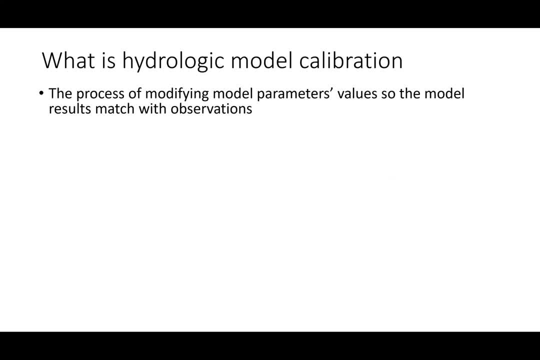 Now that we know what a hydrologic model is, let's talk about what a hydrologic model calibration is. So the process of modifying model parameter values to match model results with observations is called hydrologic model calibration. It is assumed that after we calibrate the model, the values that we get for these 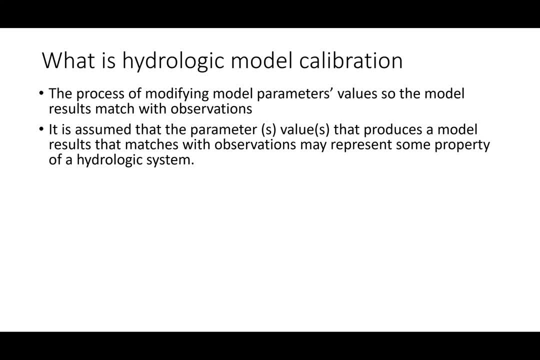 parameters may represent some property of a hydrologic system, Again using curve number as an example. a curve number does not have any physical meaning, but we do know that a higher curve number may represent an urban area. a smaller curve number may represent a forested area. So that's why, even if they don't have any, 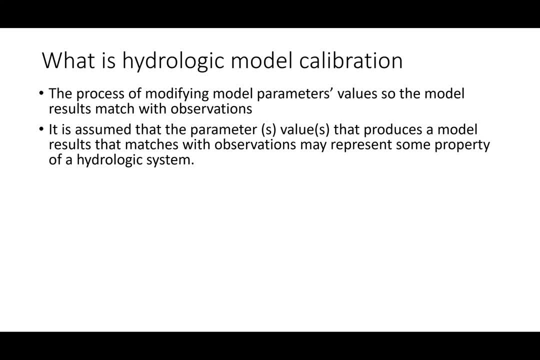 physical meaning. a good calibrated parameter may tell something about a process in a hydrologic system. Model calibration is a subjective process depending on the model type and its objective. The criteria for defining a good calibrated model may be different. So if you are using it for a design or water resources planning based, 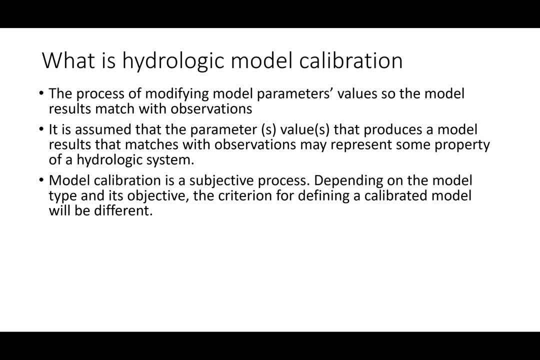 on that. the way we calibrate the model may be different. Also, depending on who is calibrating the model, we may get different results and we will talk more about that towards the end. A hydrologic model can be calibrated to match a single flux. Most hydrologic models can be calibrated to match a single flux. A hydrologic model can be calibrated to match a single flux Most. 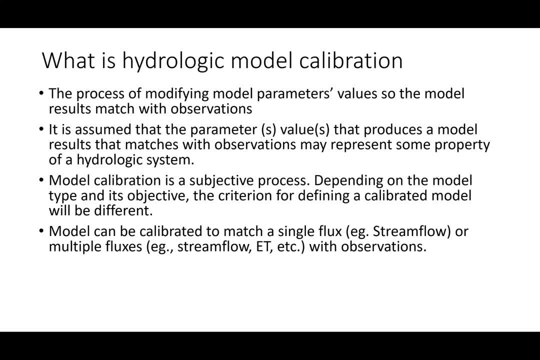 of the times, we use the stream flow at the outlet to calibrate a hydrologic model, but you can also calibrate a model to match multiple fluxes, such as stream flow, evapotranspiration, infiltration, etc. with observations. In order to calibrate a model, you need observed data, so if you have 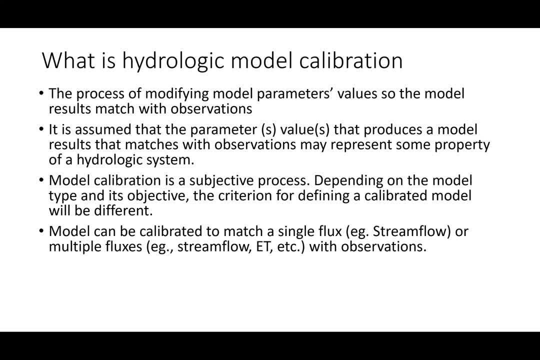 observations for multiple fluxes. you can use those for calibrating a hydrologic model. Similarly, comparisons between model results and observations can be made at single or multiple locations. So most of the times we don't have data, but if you have data at multiple locations for 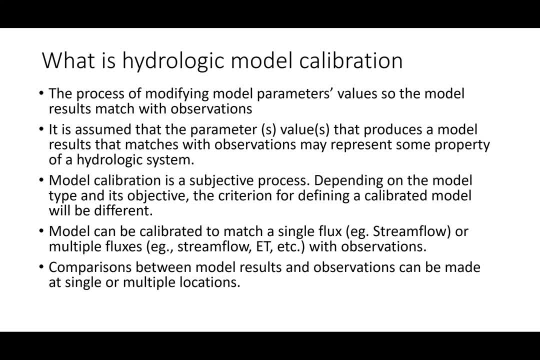 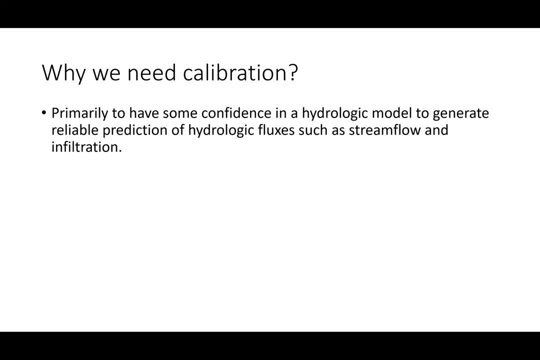 example, if you have stream flow at multiple location, you can calibrate your model to match results at multiple location. with those observations, Now that we know what hydrologic model calibration is, let's talk about why we need calibration. As I mentioned earlier, a hydrologic model may not truly represent our system. In order to have 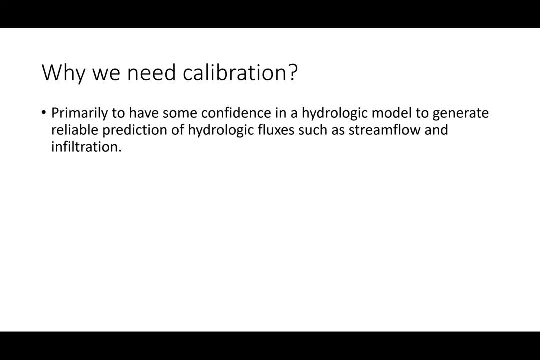 some confidence in our model to generate reliable prediction of hydrologic fluxes such as stream flow and infiltration. we want to calibrate a model, and we want a calibrated model for multiple reasons. First, we may want to use our model as a hydrologic simulator to estimate and predict hydrologic. 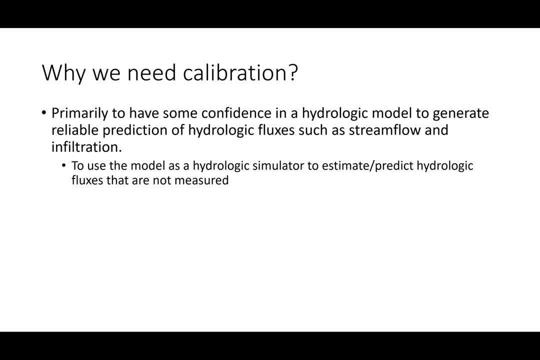 fluxes that are not measured. As I mentioned earlier, most of the times we have observations on stream flow, but we do not have any observations related to other hydrologic fluxes. So if our model is producing a good stream flow hydrograph, then we may say that the 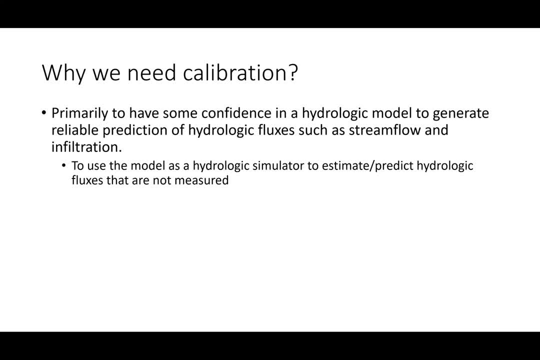 other fluxes that it is predicting may be accurate and they may tell us something about the watershed. We may also want to use our model to understand the behavior of a hydrologic system under different conditions. So, for example, if we have confidence in our model, we can learn how our hydrologic 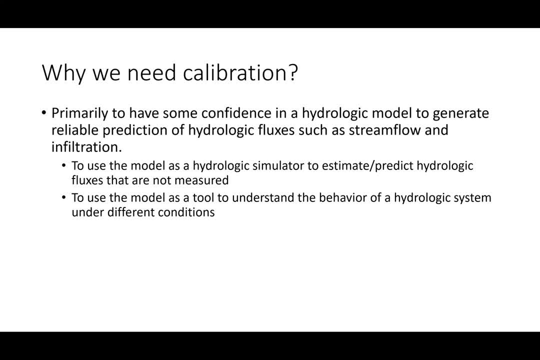 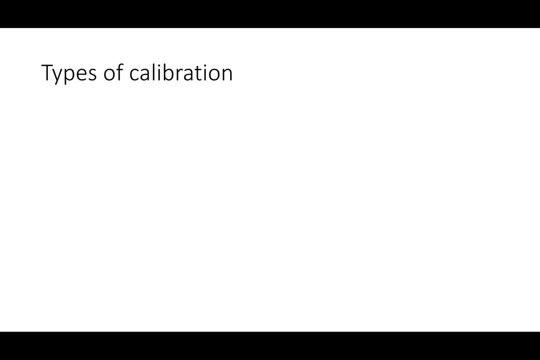 system will react to changing climate, changing land use or other human impact in the future. Now that we know what calibration is, why we need calibration, let's talk about different types of calibration. So we can calibrate a model in two ways. One is manual, so the goal here is to change. 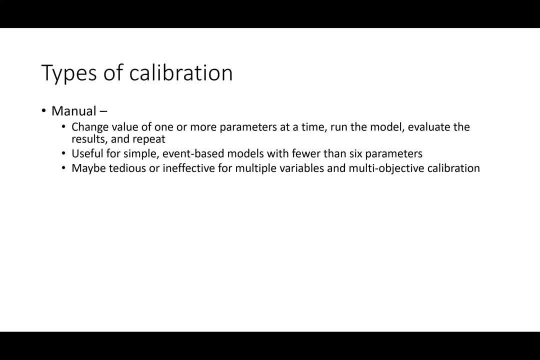 parameters to match model results with observations and we can change those parameters manually. So we can change the values of one or more parameters, run the model, compare the results. if the results match with observations and if the values of parameters make sense to us, we can stop. If not, we will continue. 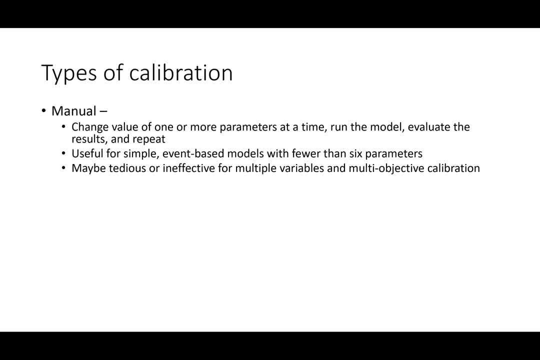 that process until we get satisfactory results. Manual calibration is good for simple, event-based model with fewer parameters. so I list six parameters here, but there is no hard rule on how many parameters, so usually less than six, are easy to handle. if you are doing manual calibration, as you can imagine, manual calibration process can. 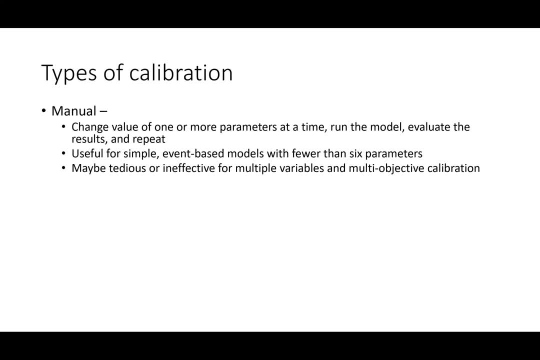 become tedious and ineffective for multiple variables and multi-objective calibration. so if you are trying to match streamflow and evapotranspiration at the same time, we will have to play with multiple parameters at the same time and this can become tedious and may not yield good results. another type of 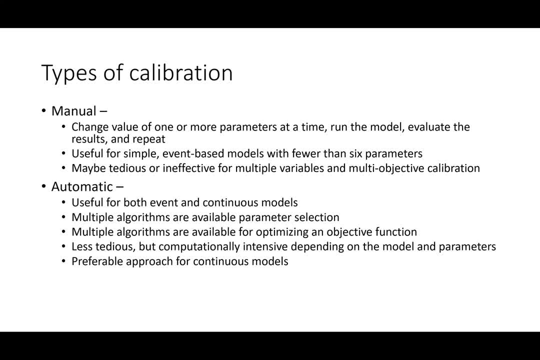 calibration is using automatic approaches, so this approach can be useful for both event and continuous based model. good thing about automatic calibration is we have multiple algorithms to select parameters to optimize objective functions, and it is very easy to use. and it is very easy to use. and it is very easy to use and it is. 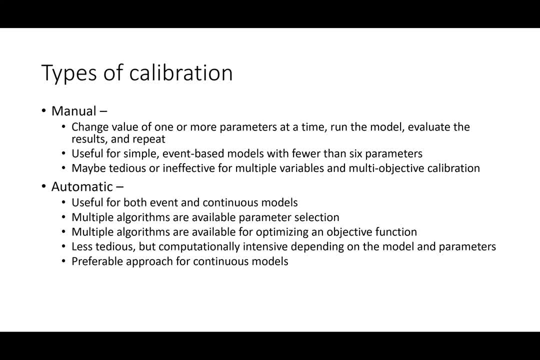 relatively less tedious, but it does require computational resources when we have a complicated model with lots of parameters. manual calibration is good for event based model. if we are working on a continuous model that has a simulation for many years, automatic calibration may be a preferable approach. but most of the times, with experience and practice, we may choose to combine. 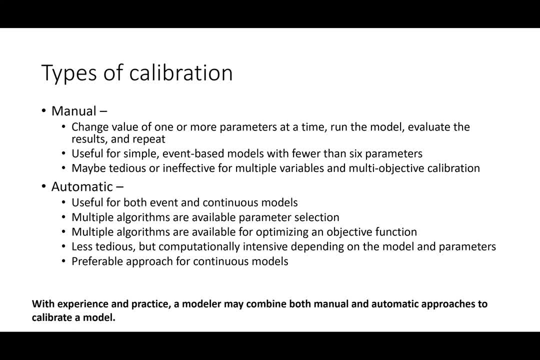 both manual and automatic approaches to calibrate a model. automatic approach is basically a computer technique, so computer may not understand much about hydrology. so if we get results, even if they are good, we still have to look at parameters and may have to tweak them manually, thus combining the automatic and manual. 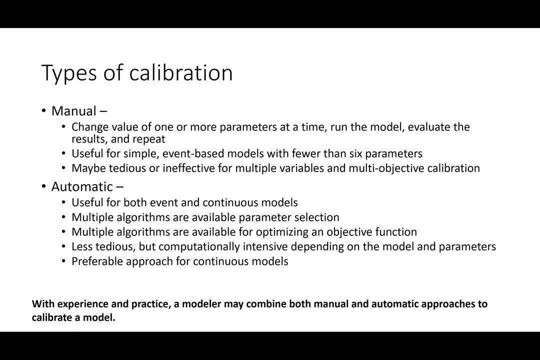 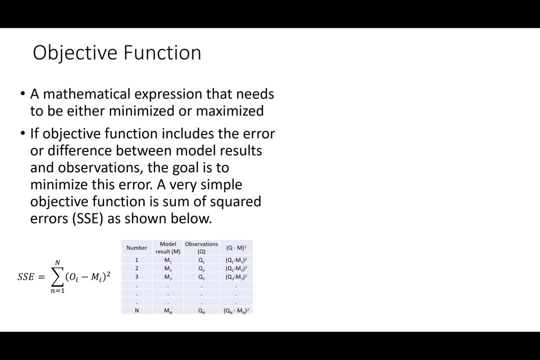 approach. when we calibrate a model using automatic approaches, we have to make selection of an objective function and then we have to calibrate the model, and an objective function is basically an expression that needs to be either minimized or maximized. a simplest example of an objective function is the: 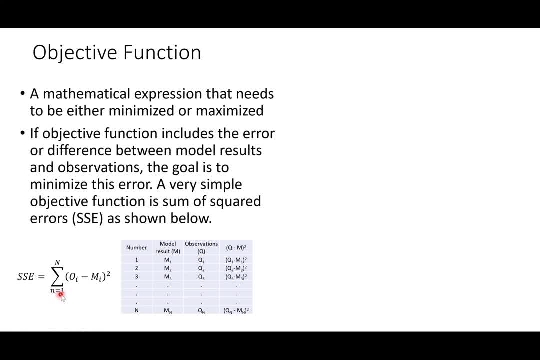 sum of squared error that you see here at the bottom. so what you see in this table is basically Excel way of calculating sum of squared error. so you have the model results, you have observations, you subtract each of them, you square them and you take their sum, and the goal here is to minimize this sum of squared errors. so, as i said, 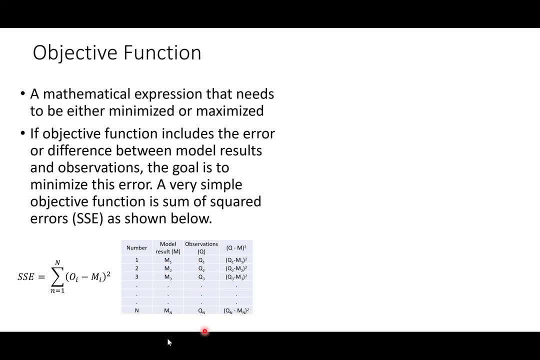 this is the simplest example. in many models you will see different types of objective functions. the common ones are nash, certainly, efficiency. in swat we also use king gupta, efficiency, percent bias and you can also use r, square root, mean square error, mean square error. so there are 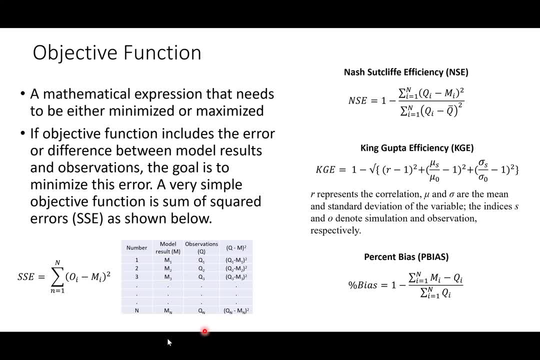 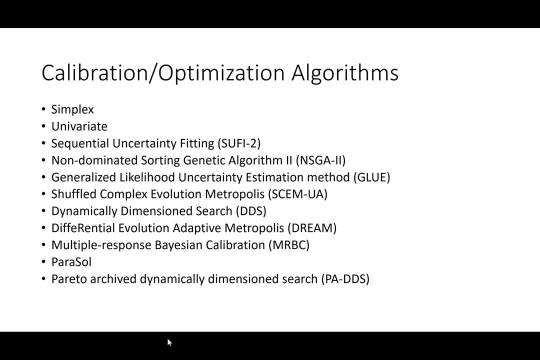 many objective functions available when we are trying to calibrate a model using automatic approach. similarly, we have multiple algorithms available for minimizing or maximizing or objective function. there is a list of some of them. we will not go into details of any of these. this is just the simple overview of some of them. i hope you will like this video and please subscribe to our channel for all the video tutorials we have. Thank you very much. 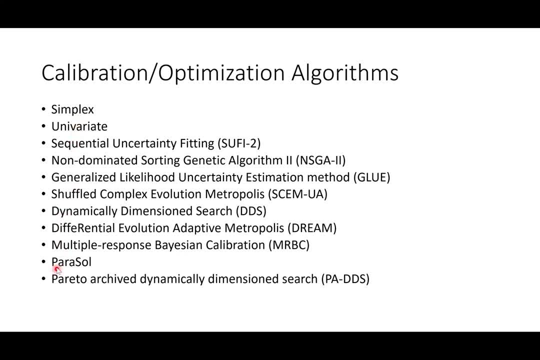 just for you to know that there are multiple algorithms available. in HEC-HMS, you will see simplex and univariate. with SWAT, you will see SUFI 2. this is used in SWAT cup and we are going to use this genetic algorithm. NSGA, you may have. 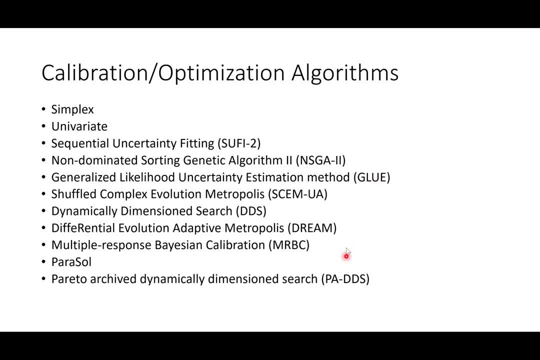 heard about glue and you may have heard about some of these algorithms that are used for calibrating a SWAT model or other continuous models. now that we have some basic information about calibration, how it is done, what is available, let's look at how to calibrate an event and continuous model. here we are using an. 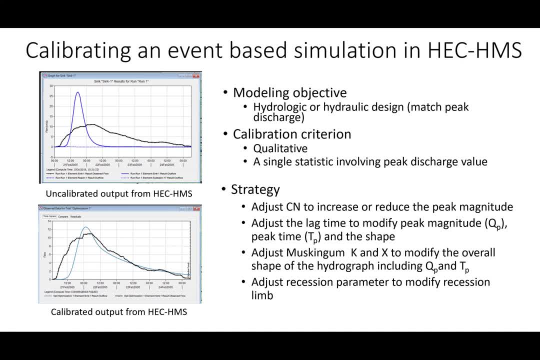 example of HEC-HMS and this is one of the models that we are going to calibrate in this module in an event-based model. most of the time, our objective is to use that HEC-HMS model as an example in HEC-HMS models, but unfortunately 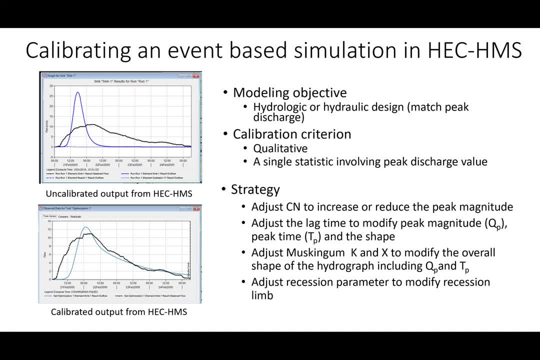 most of the time our objective is to use that HEC-HMS model as an example in an event-based model. most of the time, our objective is to use that model for hydrologic or hydraulic design, and in that case we may not be interested in matching the entire hydrograph or getting the total volume. 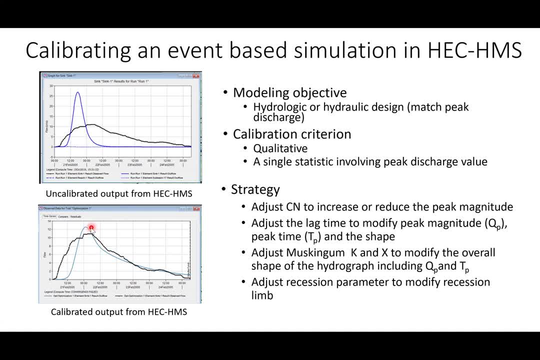 right, we may be interested in looking at the peak discharge. so what you see here is an uncalibrated model from HMS. and this is the same model, but it is calibrated to match the peak flow, so the calibration criteria can be qualitative. we can decide whether it is a good calibration or not by looking at the 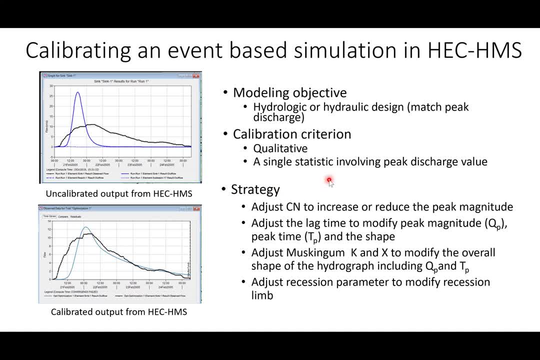 hydrograph peak or we can use a single statistic involving just the peak discharge value. so this is a curve number based model, so we can see that the model peak is much higher than the observed peak, so we can adjust the curve number. this model also uses the SCS unit hydrograph method, so we can 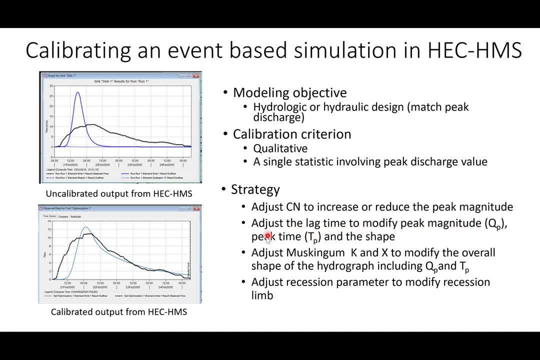 adjust the lag time to modify the peak, magnitude time to peak and shape. we can also adjust the Muskingum K and X that are used for channel routing to modify the overall shape of the hydrograph and, if base flow is included, we can adjust the recession. 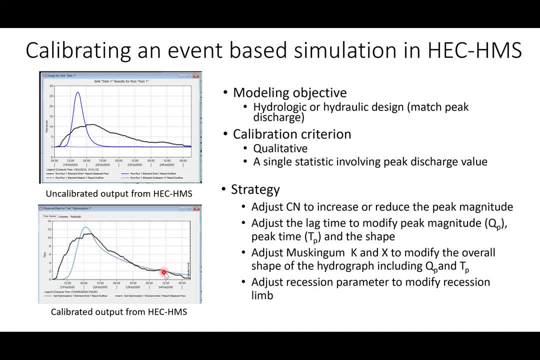 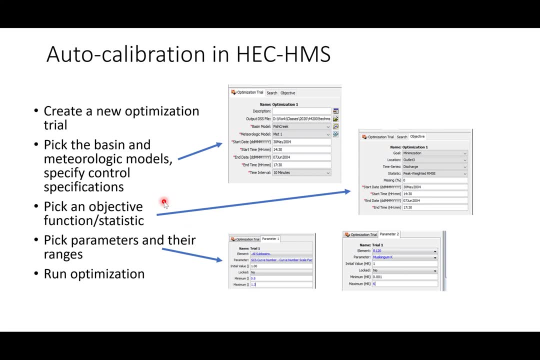 parameter to match this recession limb. so these are some of the strategies that we can use when we are trying to calibrate a HEC-HMS model manually. HEC-HMS also has routine to calibrate the model automatically. so in order to calibrate a HEC-HMS model, we have to create an optimization trial. so when we 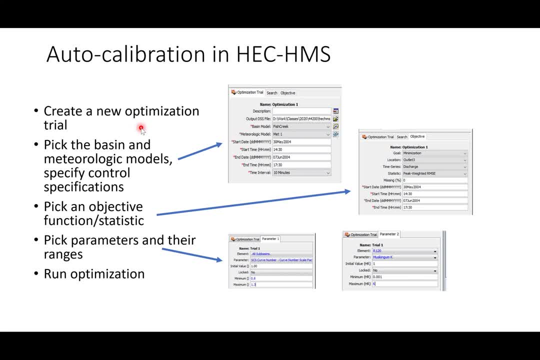 run a normal simulation. we create a simulation trial for calibration. we will create an optimization trial. after we pick an optimization trial, we have to pick the basin and meteorologic models that we want to include in our optimization trial and we specify the start date and end date time, similar to what we do in creating. 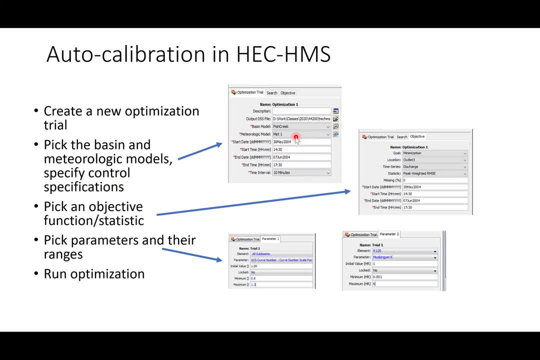 a control specification file once we tell the program what basin and meteorologic model to use. the next step is to pick an objective function or a statistic to evaluate the performance of our calibration. and finally, we have to pick all the parameters that we want to calibrate and give a range within which. 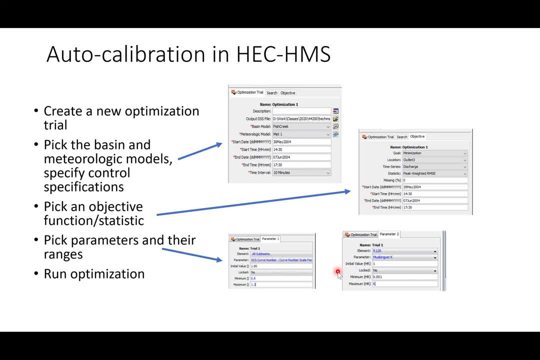 model can modify the values and then, finally, we run the optimization. So this is a simple procedure in HEC-HMS, using the optimization trial to calibrate a hydrologic model, and we will perform this process when we run the auto calibration unit in this module. 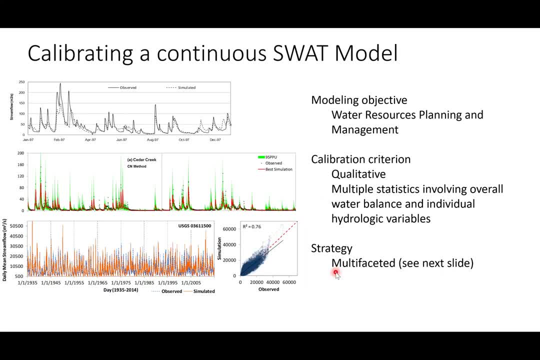 Calibrating a continuous model such as SWAT is much more complicated than calibrating a HEC-HMS model manually. Most of the times, a continuous model is used for long term water resources planning and management, and the calibration criteria it can be qualitative. 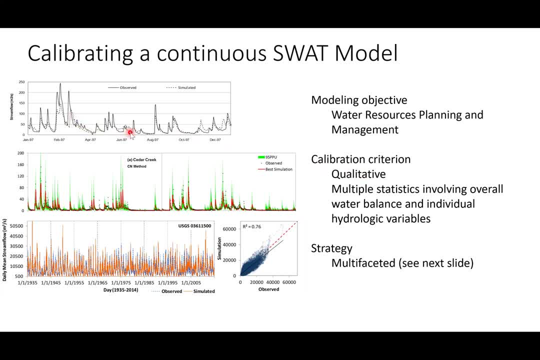 So qualitative meaning, can we look at the hydrograph and tell whether the calibration is good or not? Now, depending on how long the simulation is, it may be easy. but it may not be easy if the calibration is run for multiple years. So you can see in this one year hydrograph. 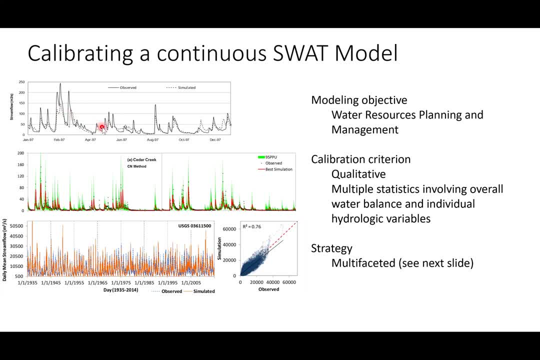 We can see the simulated output and observation and say something about the quality of calibration. but as the simulation time gets longer and longer, it is difficult to make a judgment on the calibration just by looking at the results visually. So, for example, this is a 70 year of simulation and we can hardly tell whether the simulation 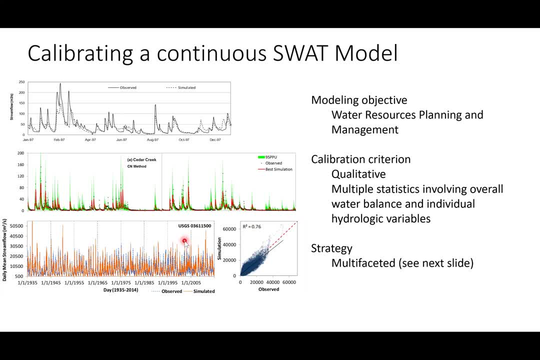 is good or not. So just qualitative Evaluation of calibration for continuous model may not be enough, and we may have to use multiple statistics involving overall water balance and individual hydrologic variables. Then what strategy we can use to calibrate a continuous SWAT model? 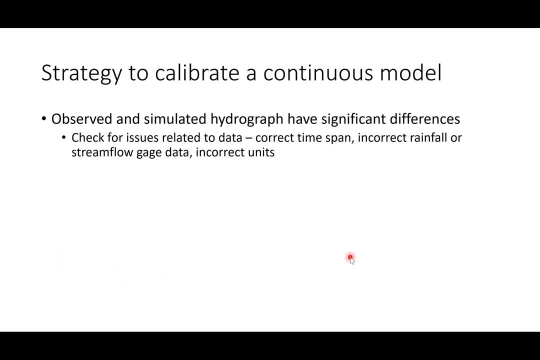 Now, depending on how the hydrograph looks, we may have to implement multiple strategies, So we may see that the observed and simulated hydrograph Have significant differences. they may look very different. If that is the case, the first thing we want to do is we want to check whether the data 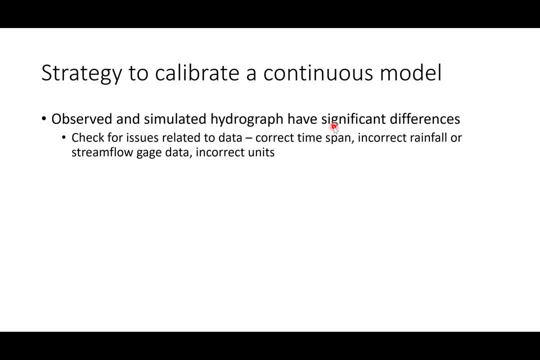 that we are using is correct. What that means is whether the observed data and the simulated data do they overlap correctly in terms of time period, Whether the rainfall data or the streamflow data that we are using. is that the correct gauge? And whether we are using both rainfall and streamflow data. 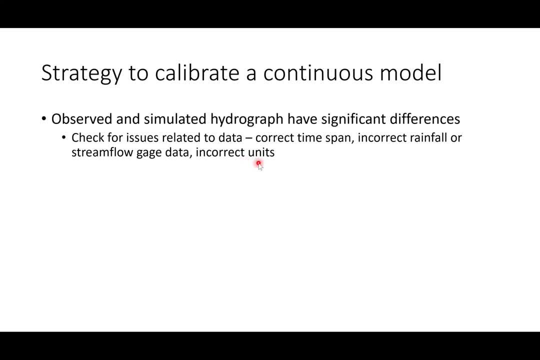 So that is the first thing we want to do. So let us take a look at the simulated hydrograph and see whether the simulated hydrograph does not match with the observed hydrograph. These are some of the things that we can check if our simulated hydrograph does not match. 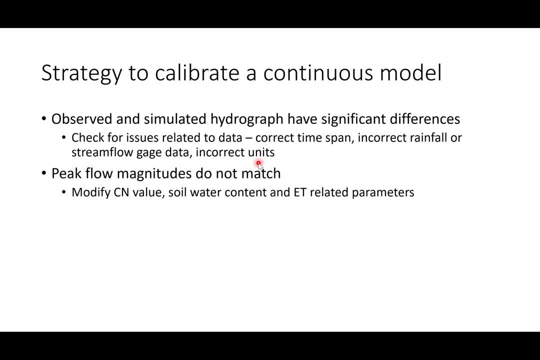 at all with observed hydrograph If the peak values do not match. so the peak has to do with how much water is running as surface runoff. So in that case if you are using curl number, we can modify the curl number. But the surface runoff is also affected by how much water is going into the soil and 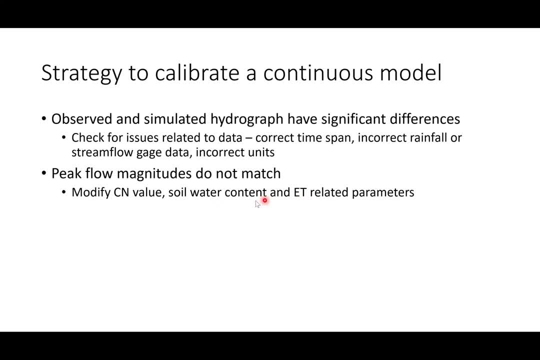 how much water is going into the soil is getting evaporated in long-term simulation so we can modify parameters associated with those processes. sometimes the peak may match, but the low flows may not match. in that case we have to look at the parameters associated with subsurface and groundwater related processes, and sometimes both. hydrograph. 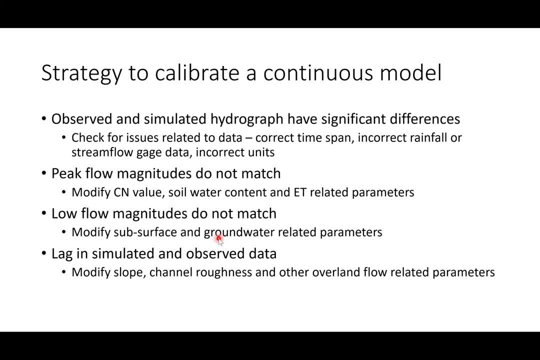 may look okay, but they may not overlap perfectly, and that has to do with water moving either slowly or too fast in our simulations. in that case, we can modify slope, channel roughness and other over land flow related parameters. so these are some of the strategies that we can use when calibrating a continuous 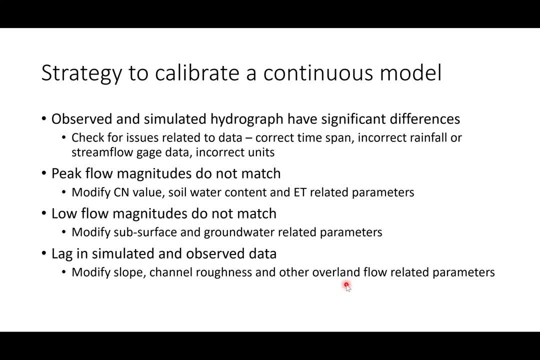 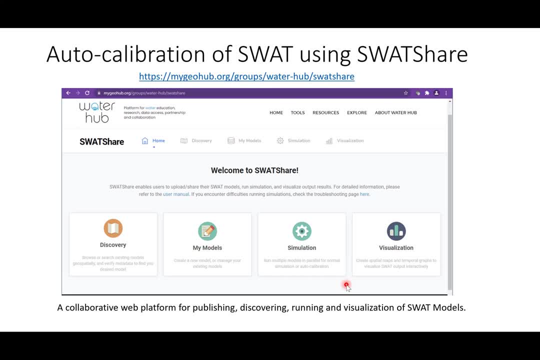 hydrologic model, and these strategies will be useful for both manual calibration and auto calibration. unlike HMS, SWAT does not have a inbuilt auto calibration functions. there are small drivers in the HMS SWAT program that apply the same. some other external software, such as SWATCup, available to calibrate SWAT. 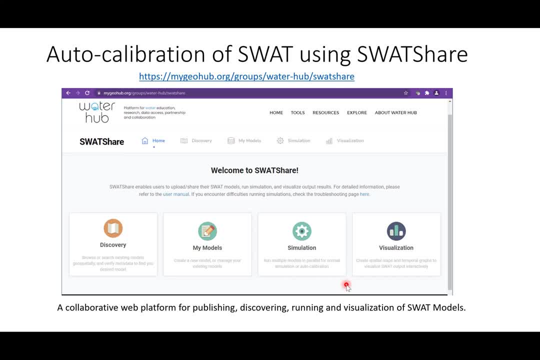 In this module, we are going to use SWATshare. SWATshare is a collaborative web platform for publishing, discovering, running and visualizing SWAT models. This is how the SWATshare interface looks and this is the link to access SWATshare. So it's freely available, but you need to have a login to use SWATshare. 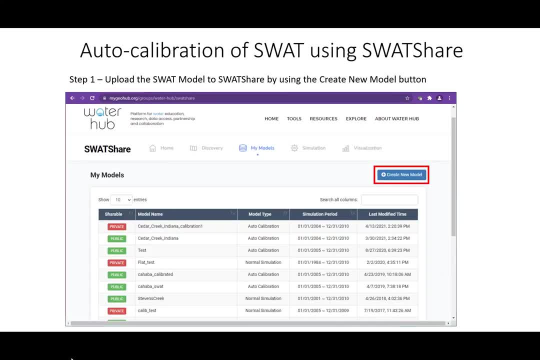 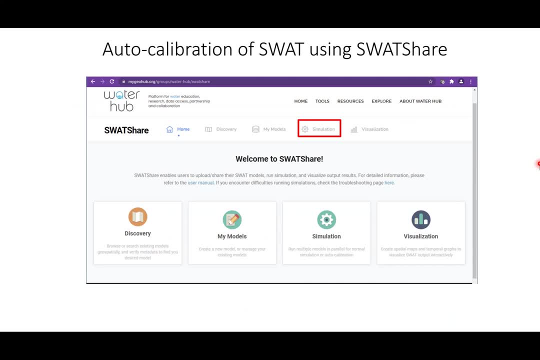 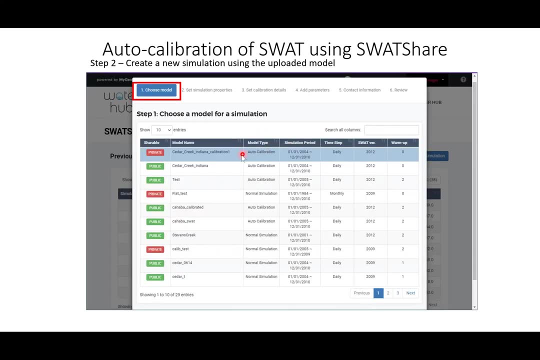 So the first step that we have to do is we have to upload our SWAT model into SWATshare. So that's our first step. After we upload our SWAT model, we have published our model in SWATshare, Then we will go to simulation and then we will pick our model for creating a simulation. 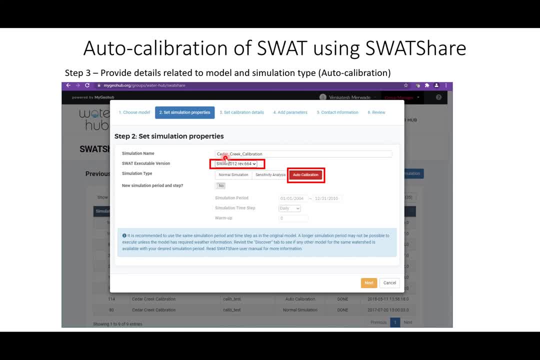 Next, We will specify what kind of simulation we want to create. So we want to use auto calibration. We have to specify what version of SWAT was used and we have to provide a name and some of the other related metadata that will be extracted by SWATshare from the files that we upload. 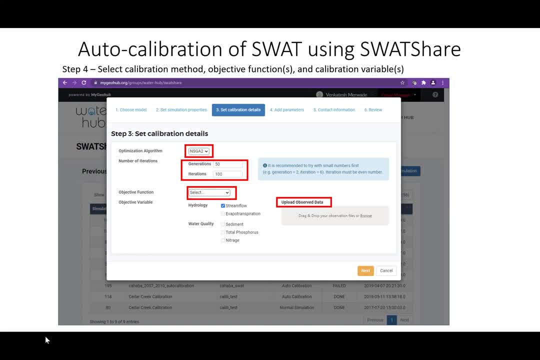 Next, we have to pick the optimization algorithms. So SWATshare currently has only one optimization algorithm, which is this NDA. This is a genetic algorithm, So we have to specify parameters associated with that algorithm. We have to pick an objective function. 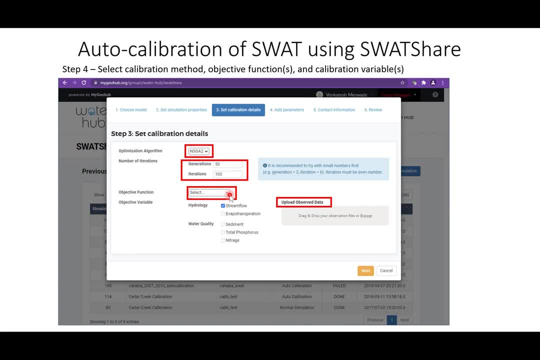 And then, since we are trying to match our model results with observed data, depending on what variables we pick for optimization, we have to upload the observed data associated with that. One good thing about calibrating a SWAT model in SWATshare is that it will allow. 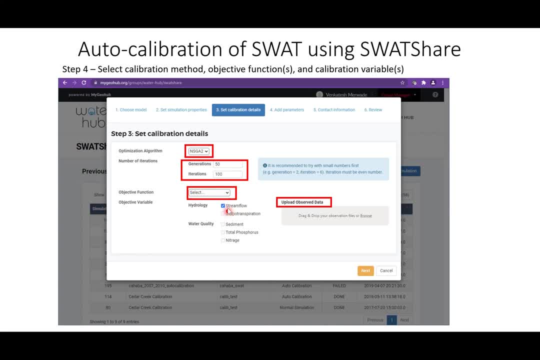 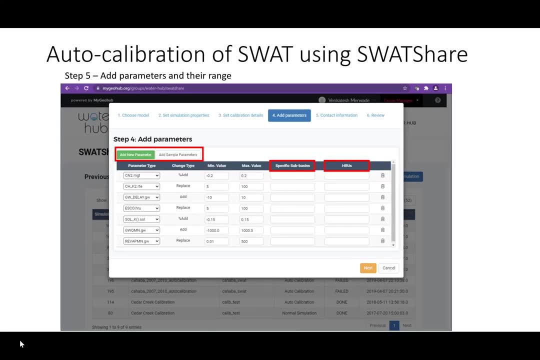 multiple variables to be optimized and also pick multiple objective functions. Next we have to specify what parameters we want to include in our calibration. So there are two ways. we can add one parameter at a time, or we can add multiple parameter by using this add sample parameter. 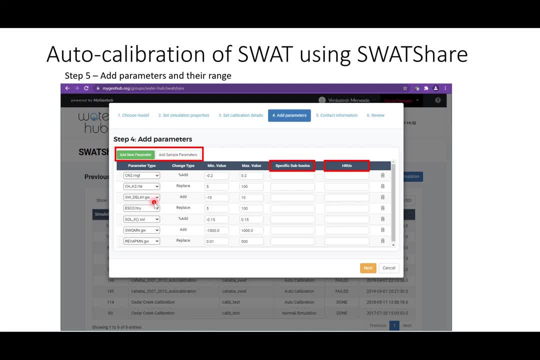 So we can add as many parameters as we want. since we are interested in just the hydrology of SWAT model, we can pick the parameters that are associated with hydrology. After you pick a parameter, the default values are populated here, which you can change. 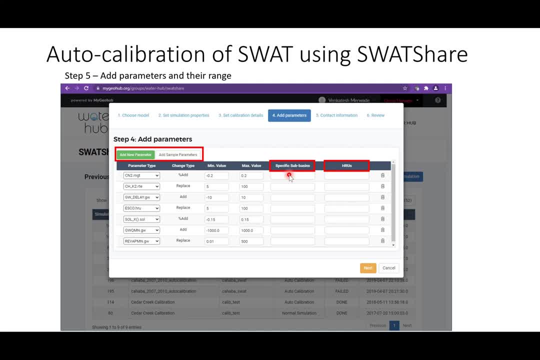 Another good thing about calibrating a SWAT model using SWATshare is that if you want to modify parameters only in specific sub basins or HRUs, you can list them here. If you don't list them, the program will calibrate parameters for all sub basins. 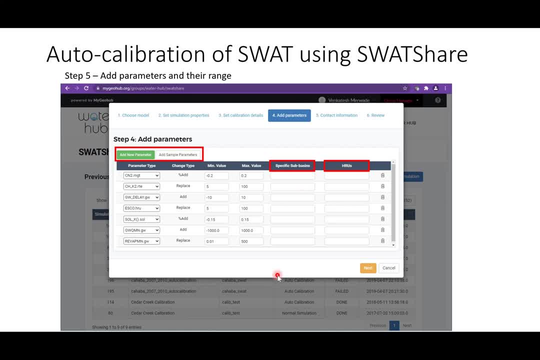 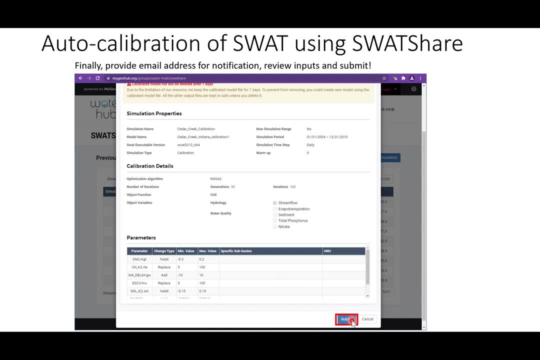 And all HRUs. Once you specify these parameters, the next thing is to review all the information that we have provided and push the submit button, and SWATshare will run the calibration And then it will email you once the calibration is done and then we can come back and visualize the results. 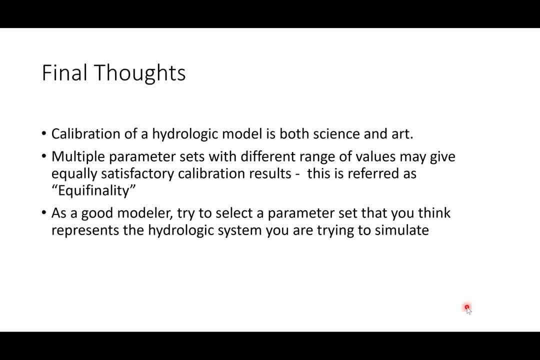 Finally, we have to understand that calibration of a hydrologic model is both science and art. What we are trying to do here is trying to match two curves. so that's where the art is, but then we have to use science to make sure that the parameters that we are getting from 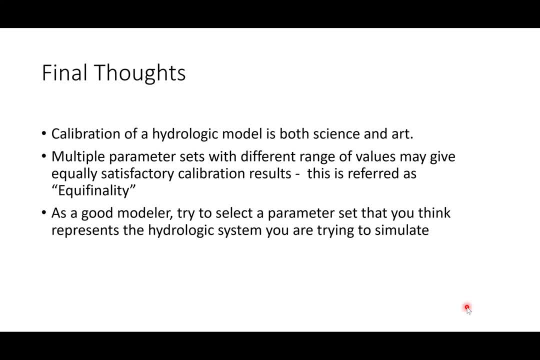 our calibration makes sense. as I said earlier, calibration is a subjective process. multiple parameter sets with different range of values may give equally satisfactory calibration results, and we call this phenomenon as equi finality. so this is one of the limitation, or you can think of as fun. 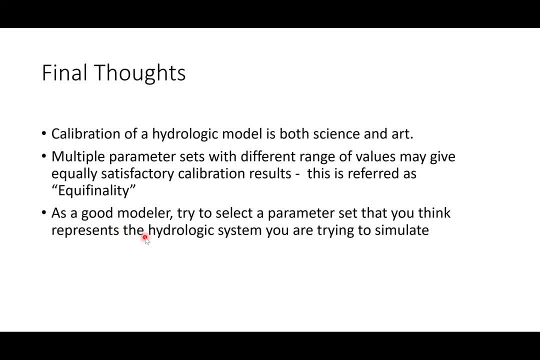 part of calibrating a hydrologic model. so, as a good modeler, we try to select a parameter set that we think represents the hydrologic system that we are trying to simulate. so I hope you got enough information to start calibrating a hydrologic model and in this module we are going to calibrate both HMS and 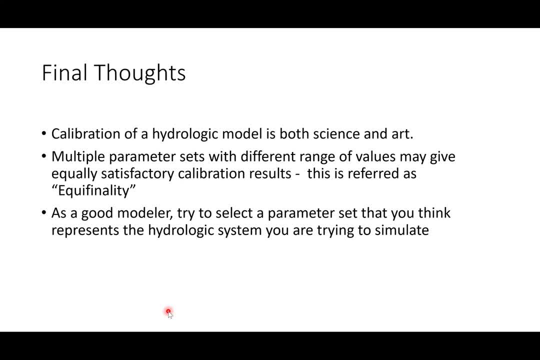 SWAT that we have created earlier. thank you,